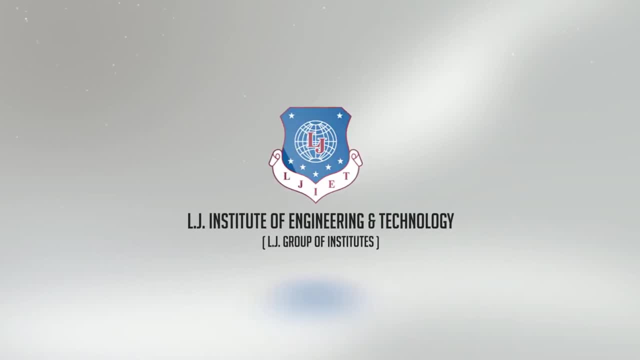 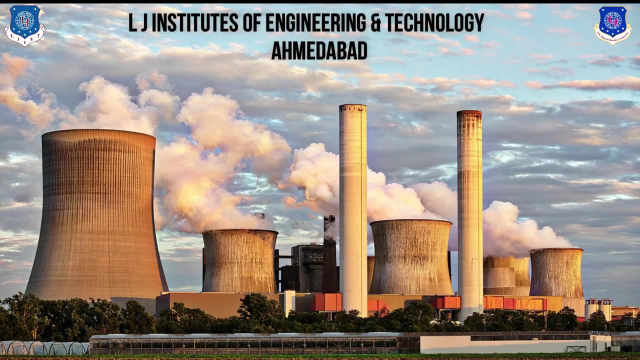 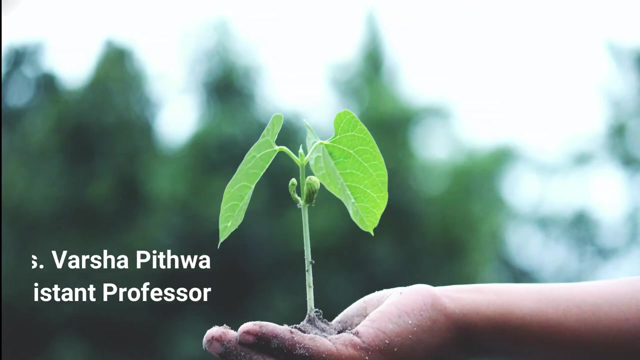 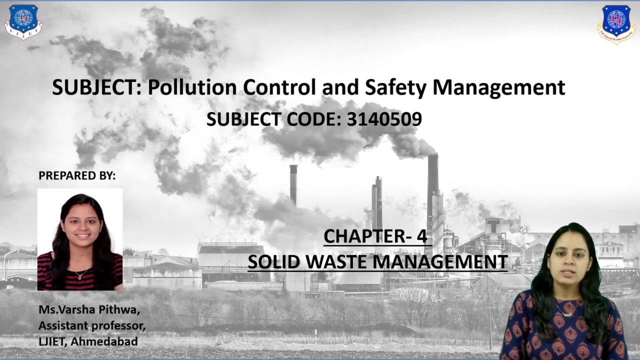 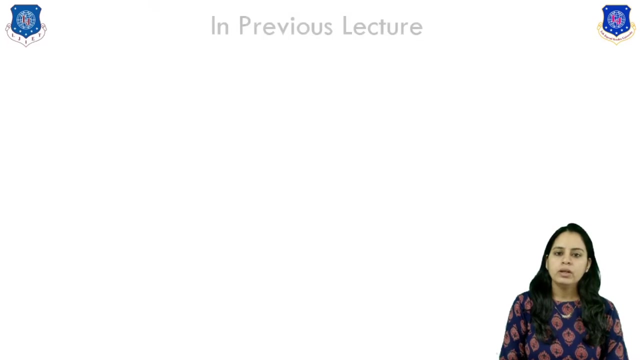 Hello students, good morning Myself, Varsha Pitwa, Assistant Professor at LJ Institute of Engineering and Technology. In today's session I will be conducting online session of the solid waste management, So start with the remaining portion Now. in the previous lecture we discussed about the three topics. 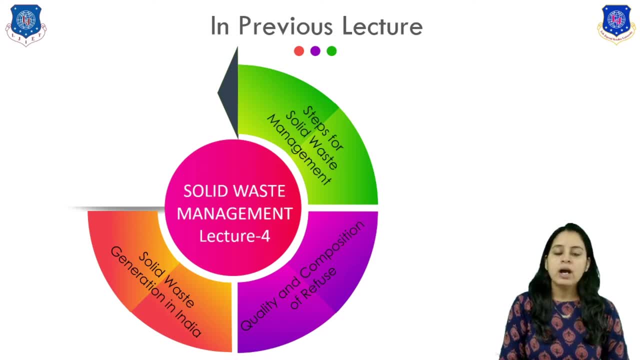 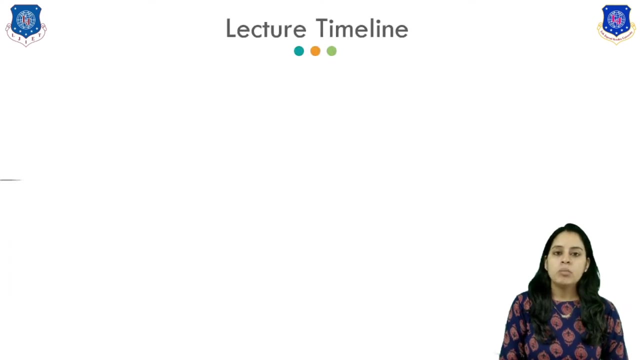 The first topic, which is the solid waste generation in India, The second topic, which is the quality and composition of the refuse or solid waste, And the third one, which is the steps for the solid waste management Right. So in the previous lecture we discussed about the steps for the solid waste. 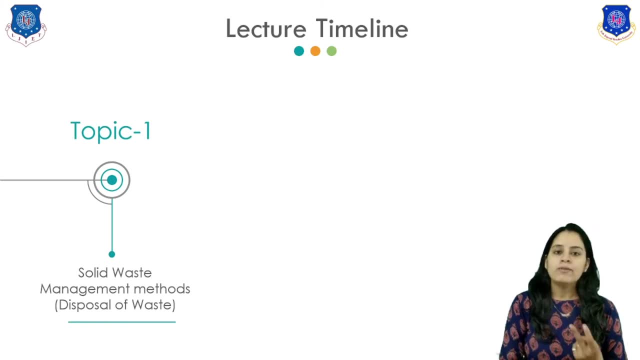 In this step: the first step, which is the collection of solid waste, And the second step, which is the processing of the solid waste. Now in this lecture we discussed about the third step, which is disposal of the solid waste. 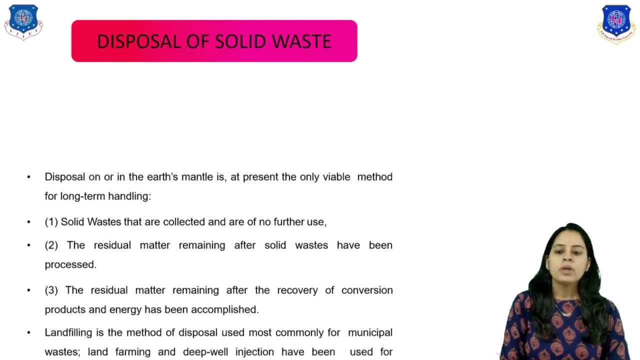 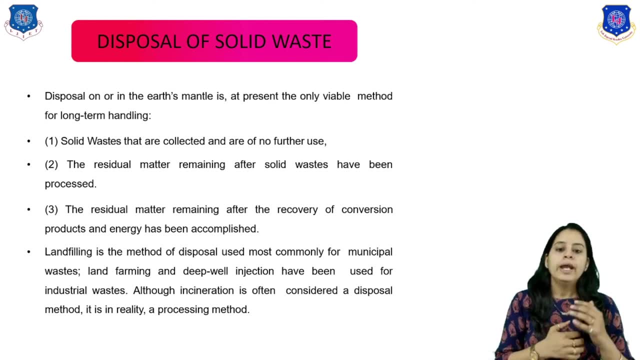 Right. So start with the disposal of solid waste. So basically, disposal, or So the disposal of the solid waste is the only method for the long-term handling of the earth's surface right. Basically, in India we are using landfilling method for the disposal of solid waste right. 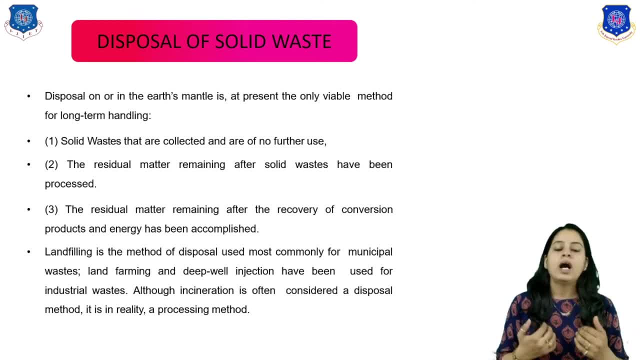 So the solid waste that are collected and are of number of further use, right. Then the residual matter remaining after solid waste have been processed and the residual matter remaining after the recovery of conservation, The product and energy has been accomplished, right. 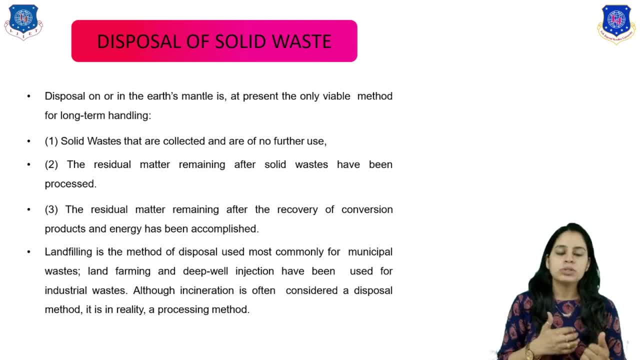 So the landfilling is the basic method of disposal used most commonly for the usable waste, Land farming and the well injection has been used for the industrial waste. Then, although the incineration is often considered a disposal method, it is reality and the processing none right. 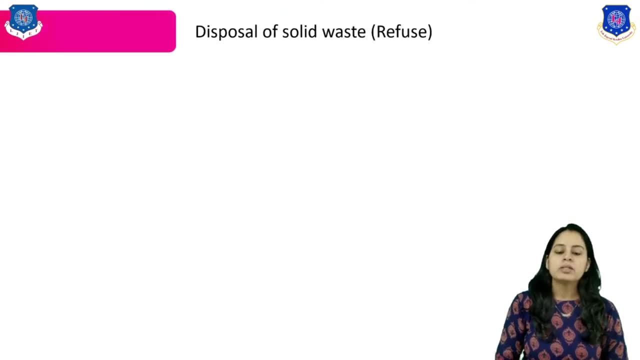 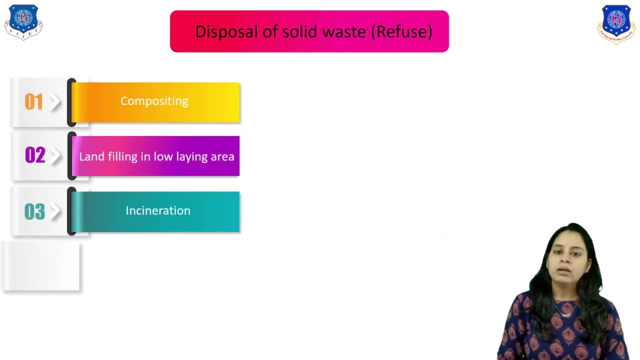 Now. so we start with the various disposal of the solid waste. Right For the solid waste method: the first method, which is composting method, the second method, which is landfilling and low laying area. it is also called sanitary landfilling. 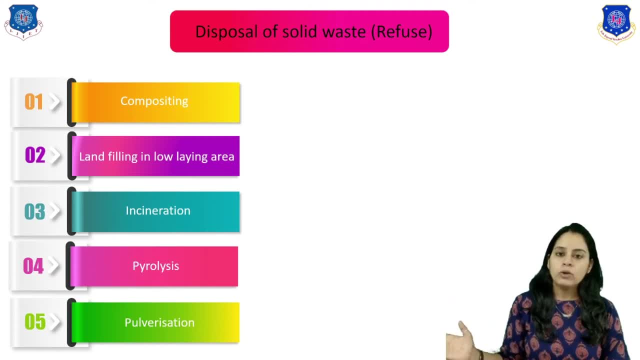 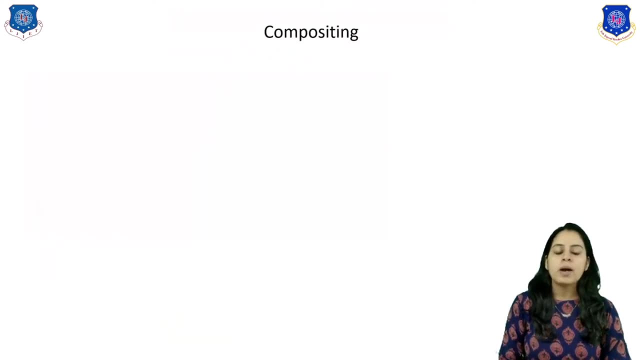 The third method, which is incineration method, then pyrolysis method and the last one, which is the pulverization. okay, So start with the first method, which is composting method. Okay, So, what is composting? 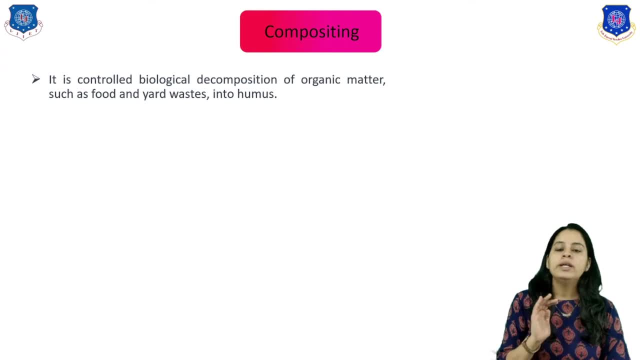 Right, So it means that it is controlled biologically decomposing. It is the decomposition of organic waste such as food vegetables than house. it is arising from the household activities, right, So it is a natural process of the rotting or decomposition of the organic matter by the microorganism under the control condition, right? 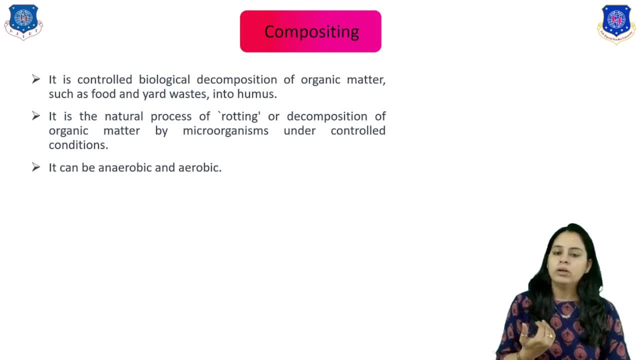 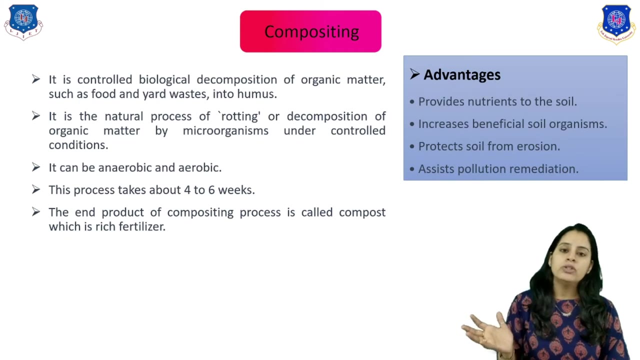 So it can be aerobic and anaerobic also, right. And this process take a four to six week And the end product of composting process is called compost, or which is which is rich fertilizer, right. So the advantage of this method, which is it provide a nutrient to the soil, right. 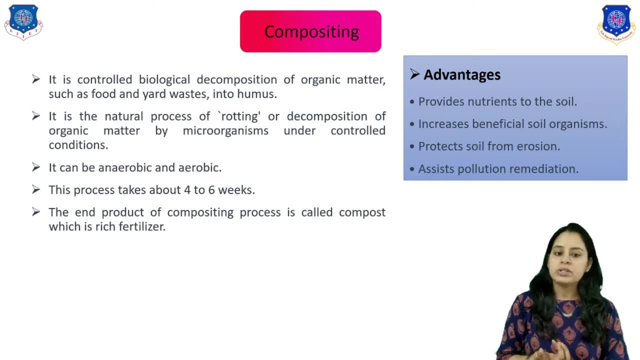 Because here, in this method, we are using organic waste right. So the it is increase the beneficial for the soil organism, then it protects soil from kerosene, then it assist for pollution remediation. right Now for this. 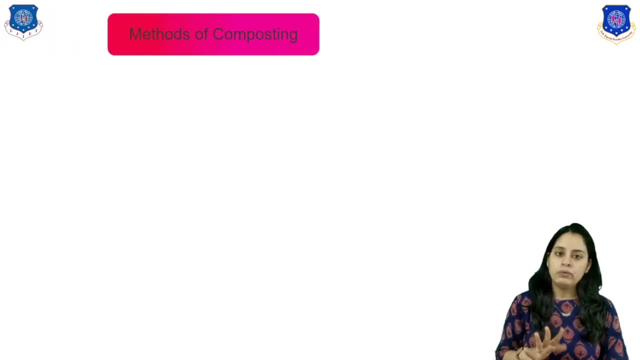 Okay, Composting. There are again. they are classified in three methods. The first is composting by trenching, then open-withdraw composting and the third one which is mechanical composting, right, So in this method, the first one, which is composting by trenching, 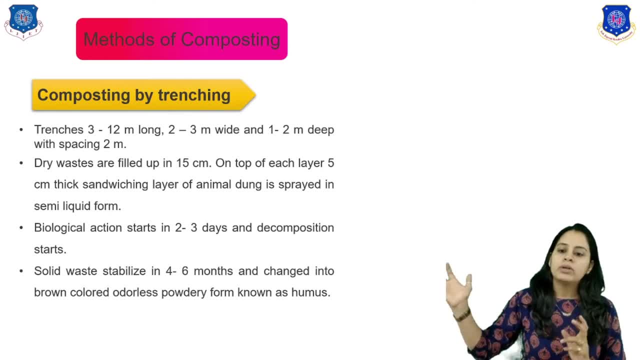 So how it is done. So for that, first of all, the trench, the size of the trench, are that right? It is three to twelve meters long, then two to three meter wide And one to two meter deep, and the spacing, which is two meter right. 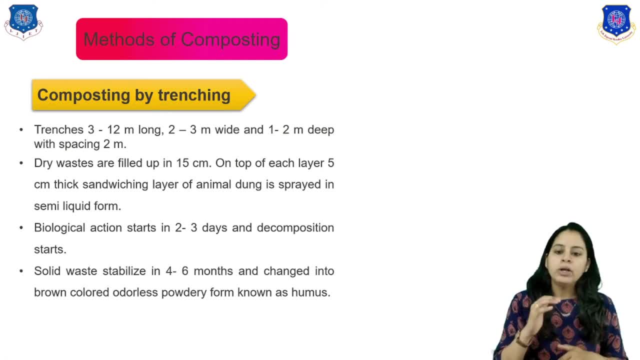 So the dry waste are filled up into the fifteen centimeter, Then one top of each layer. five centimeter thick sandwiching layer of the animal dung is sprayed on the semi-liquid form And biological action, starting two to three days and the composition decomposition will be started. 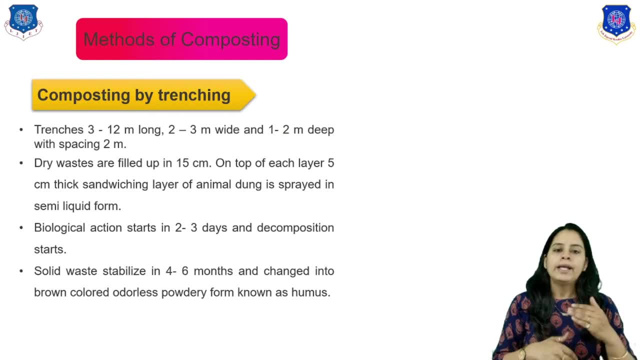 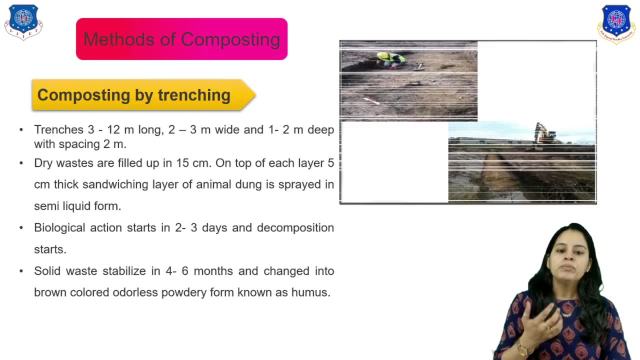 Then solid waste which is stabilized in four to six months And change into the brown color odorless powdery form It is known as a humus right. So here on screen you can see that the examples or the figure of the composting by trenching are that: 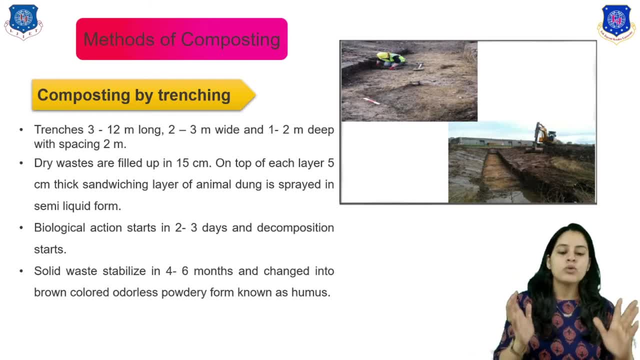 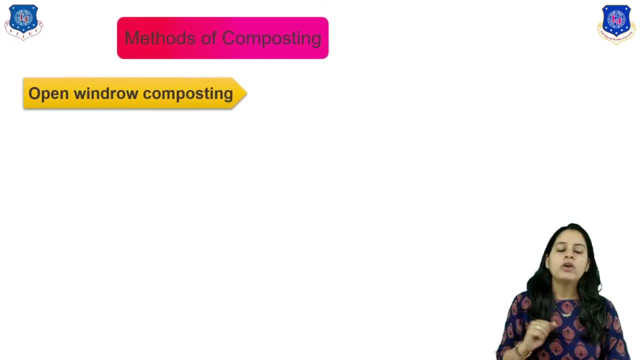 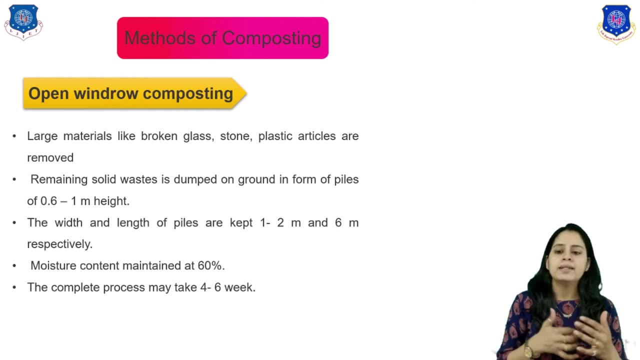 Here you can see that the trench for the composting method. the trench are that right Now, the second method, which is open-withdraw composting, It is that the large material, like broken glass, is that Stone, plastic articles are removed. 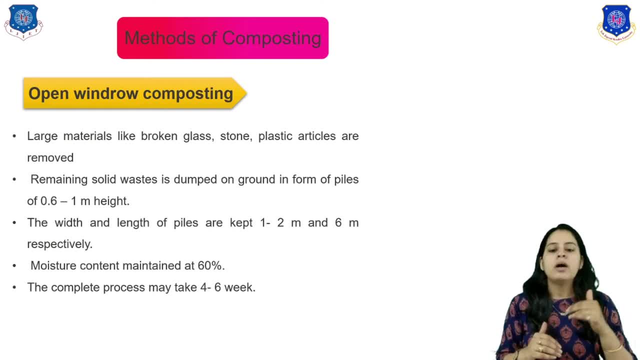 Then remaining solid waste is dumped on the ground in form of the piles of point six to one meter high right. The width and length of the pile are kept, with width equal to two meter and six meter respectively. Then the moisture content is maintained at sixty percent. 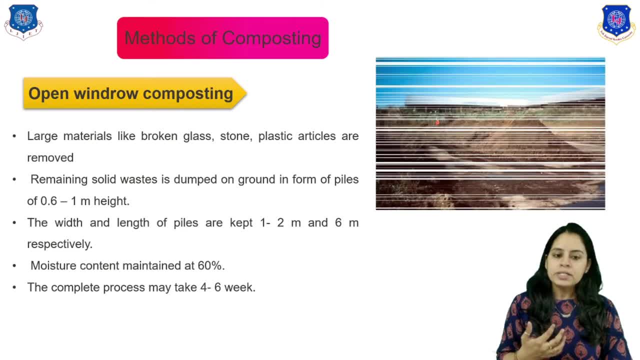 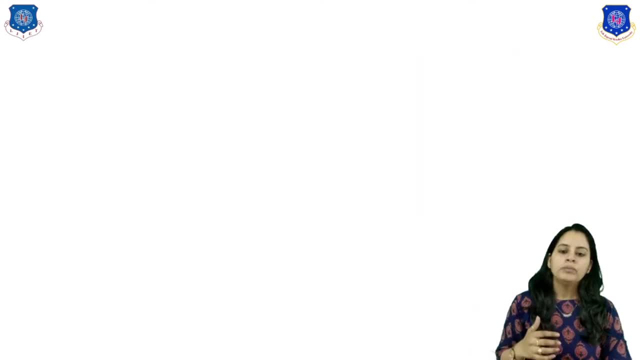 And the complete process will take a four to six week. right, Okay, Here on screen you can see that the open-withdraw composting, But the open-withdraw composting method, are that Okay? Now the third method, which is mechanical composting. 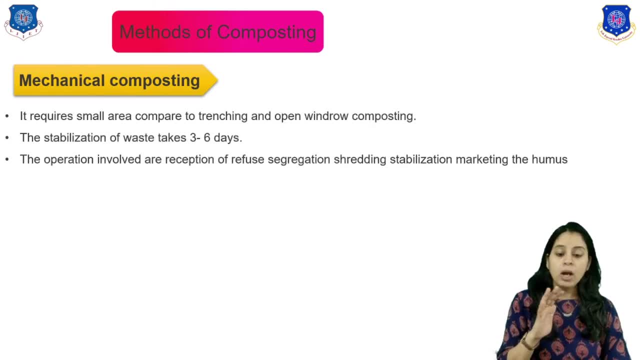 So it requires small area compared to both method- open-withdraw- and the composting method- Composting by the trench method And the stabilization of waste, which requires three to six days, And the operation involved in the reception of the refuse, The segregation, shredding, stabilization and then marking the compost right. 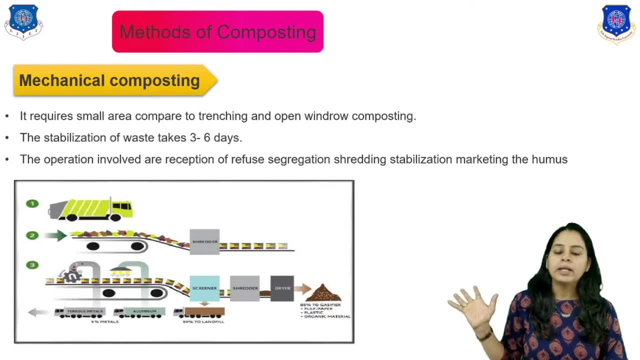 Okay. So here on screen you can see that the mechanical composting method are there For in this mechanical composting operation, which is the segregation and shredding, Okay, Then the stabilization, Okay. So for the for this segregation purpose, we are using built conveyor. 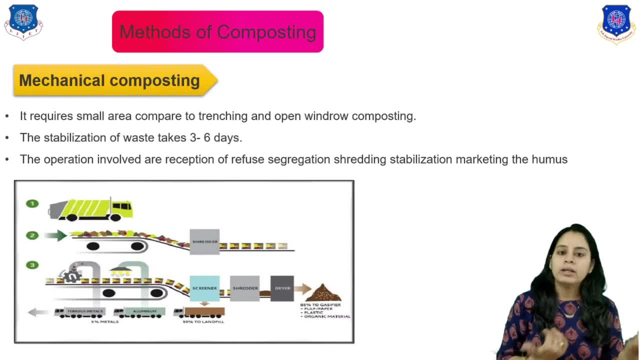 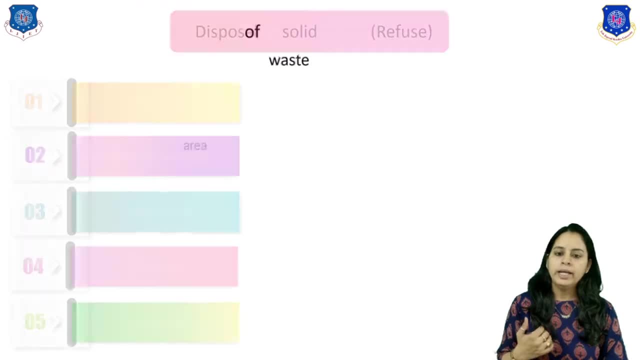 Okay, Here on the screen you can see that the built conveyor are used for the segregation of the waste, Okay, of the waste right, okay. so this is the first method, which is composting method, right now. the second method, which is landfilling in the low laying area, it is also called sanitary landfilling. 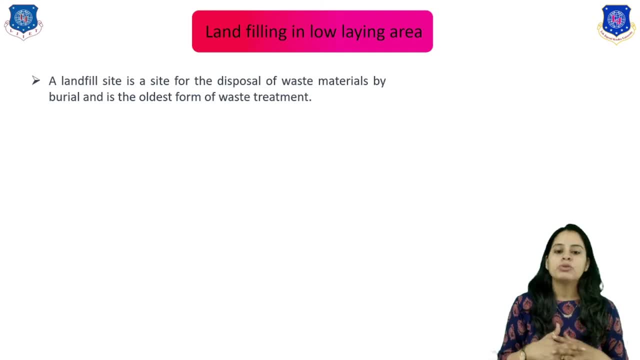 right. so a landfilling site is a site for the disposal of waste material by murate and it is the oldest form of the waste treatment right. so the in this method waste is directly dumped into the uh mining voids or the borrow beds right and the disposable waste is compacted and converted. 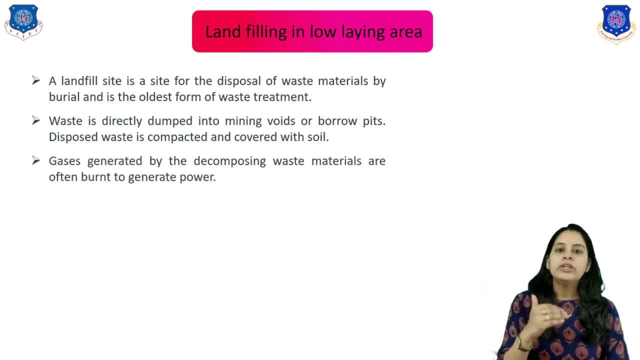 with the or the cover with the soil. so the gas is generated by this method, by the decomposition of this waste material are often burned to the generate power and the landfilling can be done by the three method: the trench method, area method and the third one which is ground method right 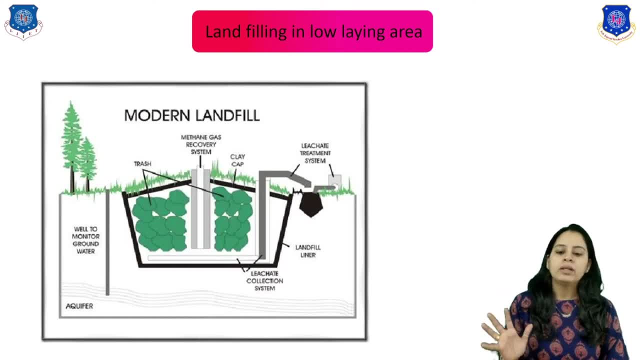 okay, here the modern landfilling methods are the figure which is given. so here you can see that the clay tap are there, then grasses are there, after that the inland filling method, the leachate which is generated, right. so here you can see that the leachate collection system are also given, because this leachate 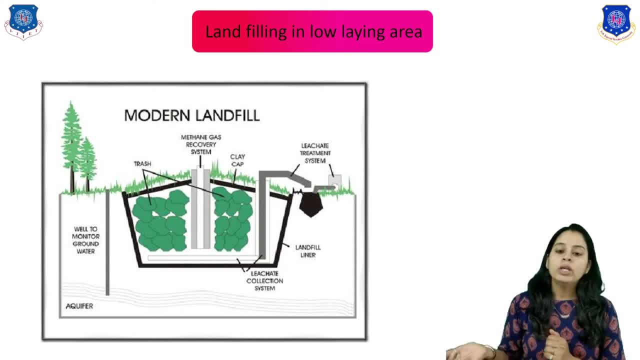 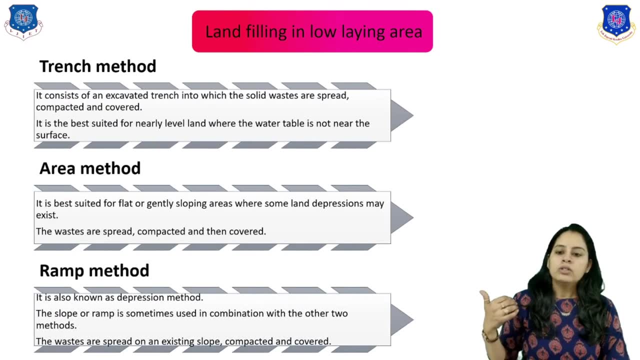 which goes to the ground water. they pollute the ground water. so here, the leachate collection method. are there right? okay, so the first method, which is trench method. so it consists of an excavated trench into which the solid waste has spread, compacted, and the cover. it is the best suited for nearly level land and where the water table is not. 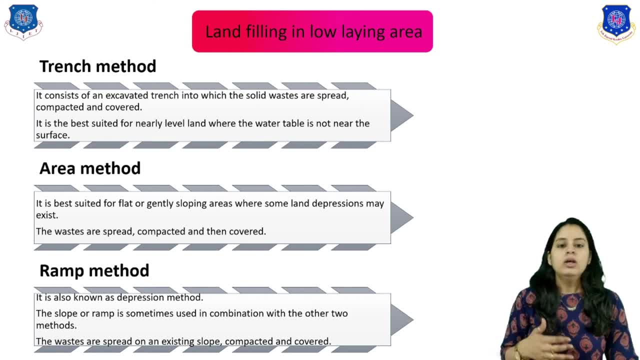 near the surface. okay. the second method: in this method it is based, suitable for the plant, or generally slowly ground where some land discretion may be exist. okay, the waste are sprayed, compacted and they cover right. and the ramp method. in this method it is also known as the depression method. 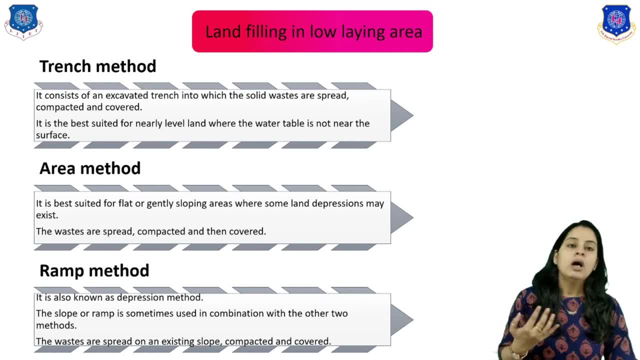 the slope or a ramp is sometimes used in the combination with two method and the waste is against. spread that straight of the existing slope, then compacted and be covered, okay. so major difference between these. in the three method, which is the place for the drench method, the it required. trench, then in area method it is a spring method, okay. so for the trench method, please do add a detergent and keep out. hey, you can put in the soil if you want, so that the soil, you can see the soil. okay, and so there is some more in the second method, okay, so the third method is in the area method then. 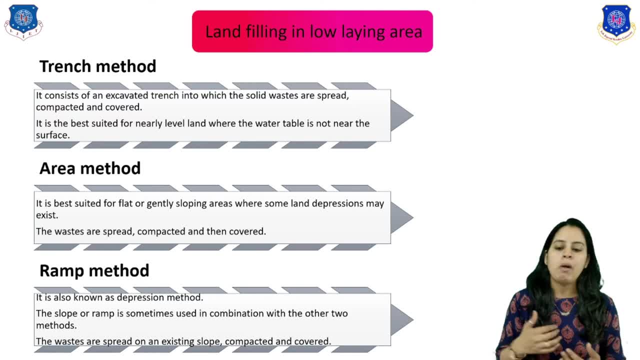 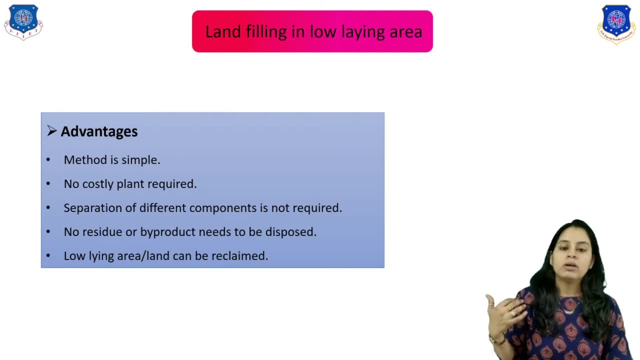 on the flat ground and the ramp method. in this method, the slope is required, right. so this is the main difference of this three method. okay, advantage of this method, which is the method is very simple method, then no costly plant which is required. then separation of different component. 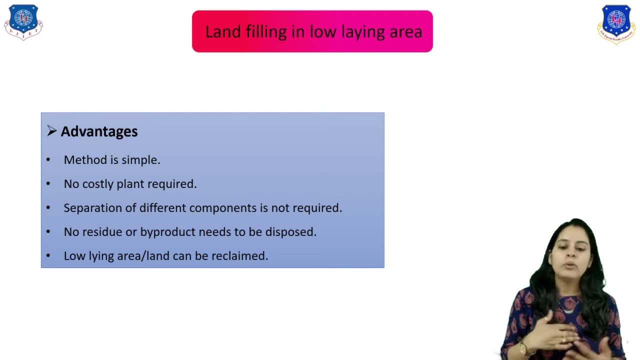 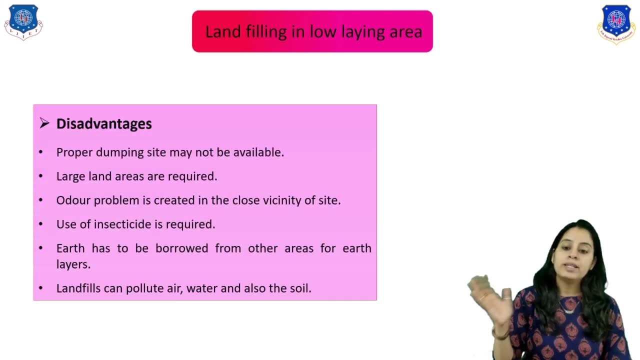 is not required, then no residue or byproduct need to be disposed of and the low laying area it can be reclaimed right now. so this third disadvantage are also there. okay, so the proper dumping site may not be available, then large length area will be required. then order problem, then use of the. 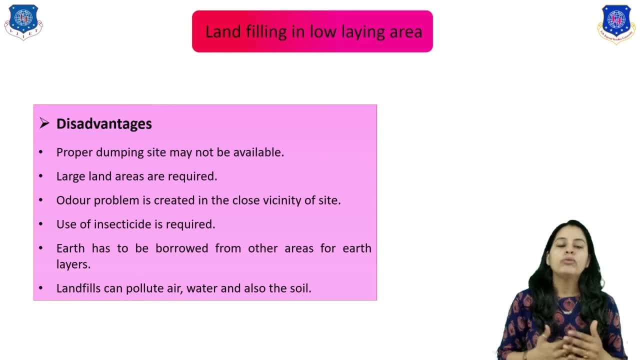 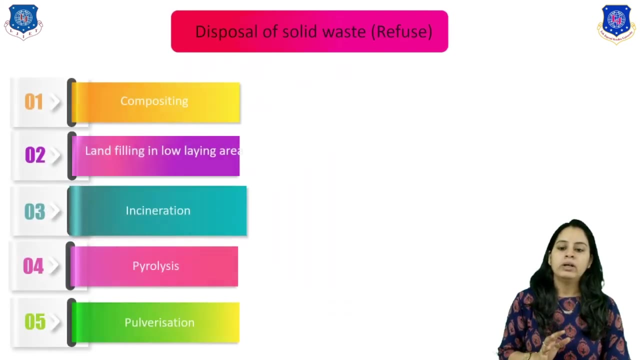 insecticides is required, then earth has to be borrowed from the other gases for the earth layer. and the last, which is landfill: it create a pollute, it can pollute air, water and also the soil, right, okay? so this is the land filling method. now the third method, which is incineration method. okay, incineration method. 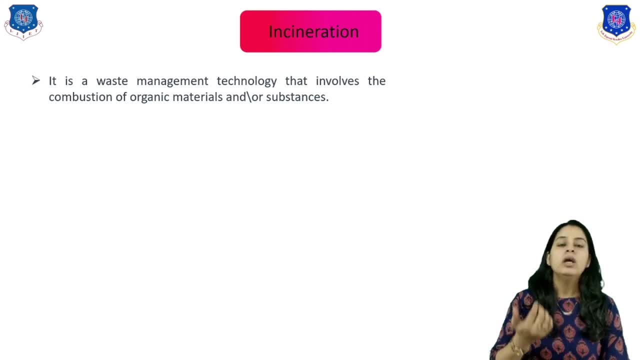 it is a waste management technology that involves the combustion of organic waste material. right, it will carry the high temperature, or it required high temperature, and the waste material is converted into the airs, then foul gases and the particulates and the heat. okay, the type of incineration, which is a moving rate incineration that. 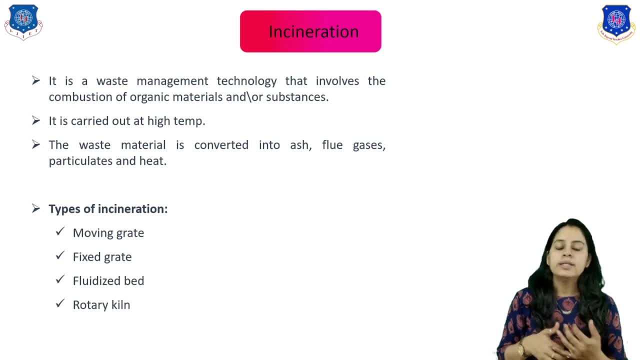 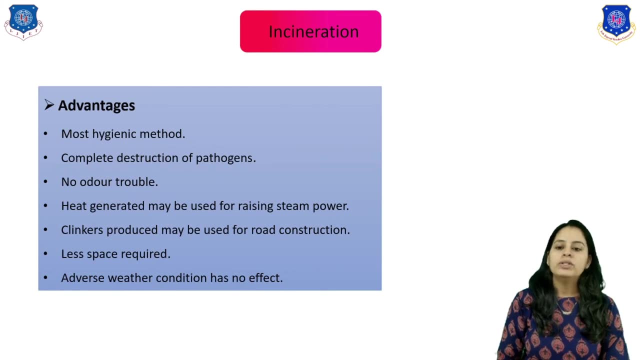 will be used for the incineration of the land will be used for the incineration of the land: fixed grade incineration, then fluidized bed incineration and the rust which is in the rotary cave. right so the advantage of this method, which is it is the most hygienic method, right then. 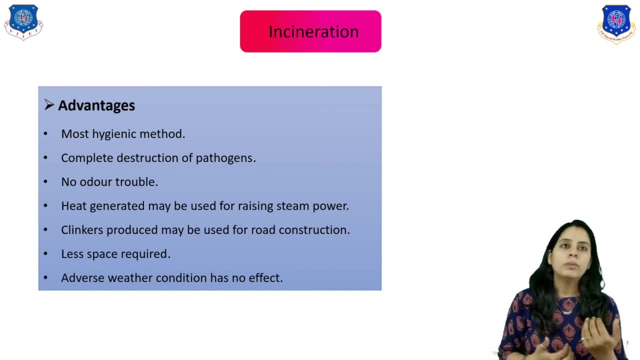 complete destruction of the pathogen and no order problems are there. the next is heat generated can be used for rising the steam power. okay, handling curves produce may be used for the road, road construction also. then lay space is required and the adverse weather condition has a no effect. okay, so there is. 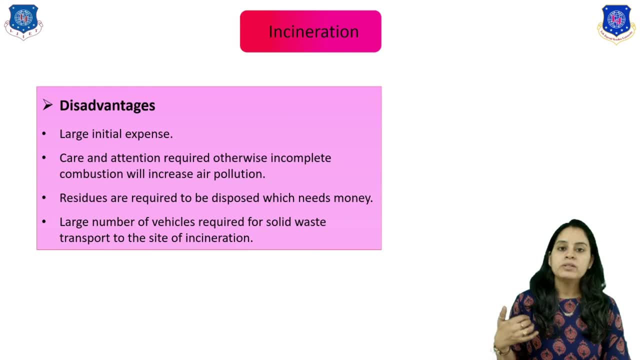 advantage of this method, which is large initial expense- uh, because it required a cough sleep plant and care and attention required, otherwise incomplete conversion will increase the air pollution. right then, residue are required to be disposal, uh, which needed the money. and the last one, which is large number of vehicles required for solid waste production of the land. so the 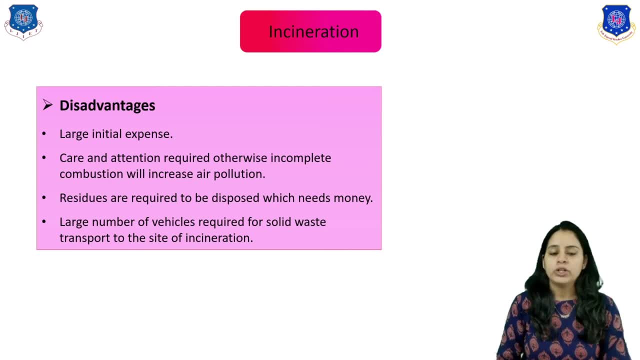 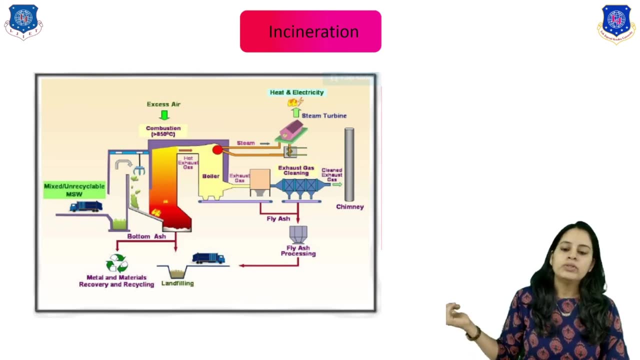 it transport to the side of the incineration, right? so this is the disadvantage of this process. okay, here the plant. are there? basically the waste which is goes to the. here on screen you can see that the waste which is transported and the waste, whole waste, which is storage in the container. 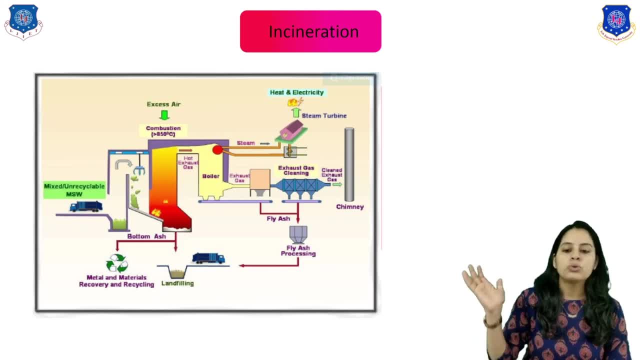 after that, some part of the waste which is goes to the combustion process and some part of the waste which is goes to the recovery and recycling process, right and the combustion process. the waste which is the combustion and the air or the excess air are the heat will be produced and this heat 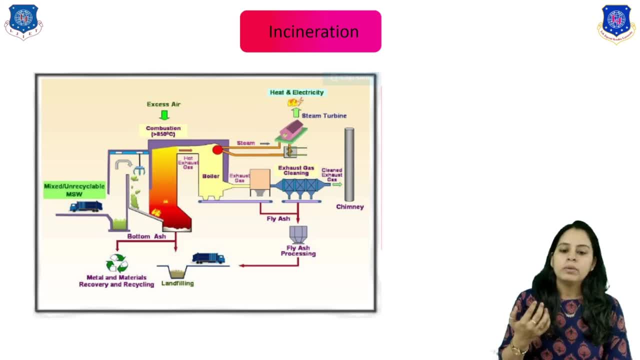 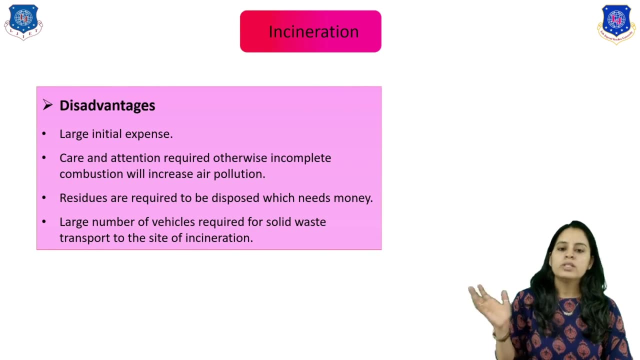 will be used in the boiler to generate the steam, right, and the last one, and the some by-product, residue product, are also generated, which is as, and these by-product, which goes to the landfilling process, right, okay, okay. so this is the all about the incineration process. now the next one, which is the pyrolysis. 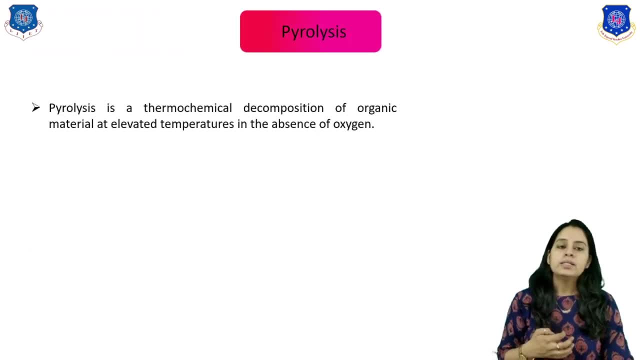 okay, so what is pyrolysis? it means that it is the same process, same as the incineration process, but it is a thermo-chemical decomposition of organic material right in absence of the oxygen, and it required temperature about 1200 degree celsius to 1000 degree celsius. it involved the 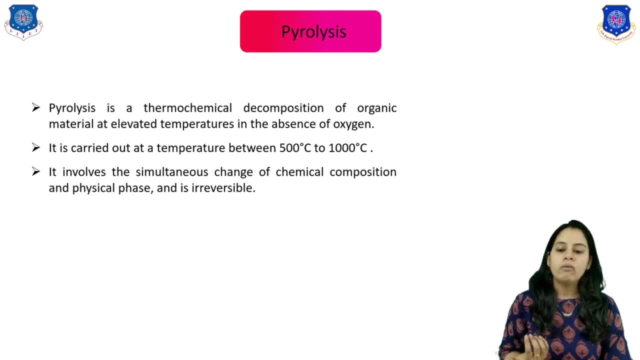 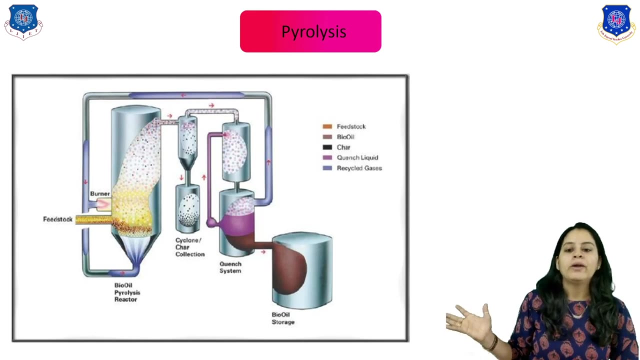 simultaneous change of the chemical composition and physical phase and it is irreversible. right and external heat source is employed and it killed gaseous and liquid and solid fractions. okay, so here on screen you can see that the plant of pyrolysis are there. okay, the first of all, the material or solid waste which is inserted or goes to the pyrolysis.